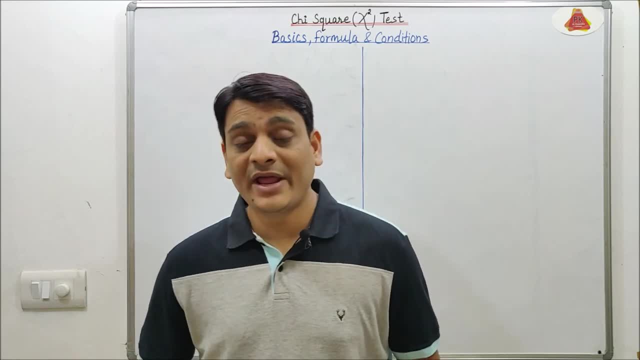 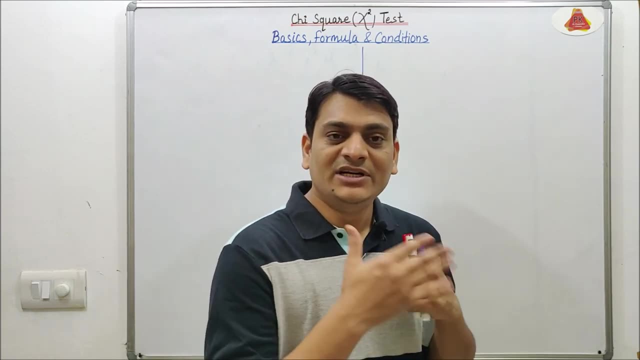 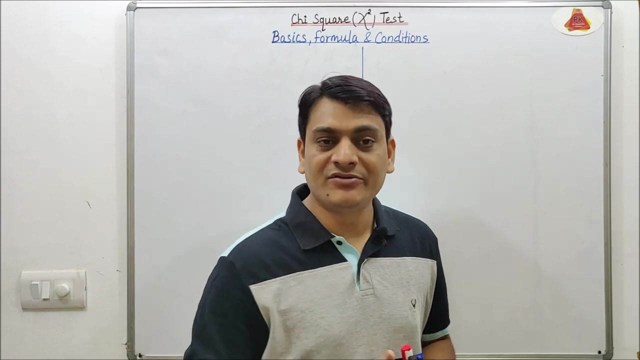 I am going to discuss about basics, formula and the conditions for applying chi-square test. This chi-square test is sometimes also pronounced as chi-square test. This will be divided into various parts, so in next part I will discuss about applications of chi-square test. then in subsequent part we will discuss or we will solve some questions related to. 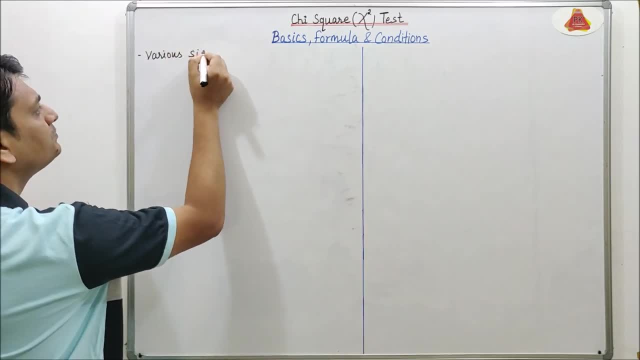 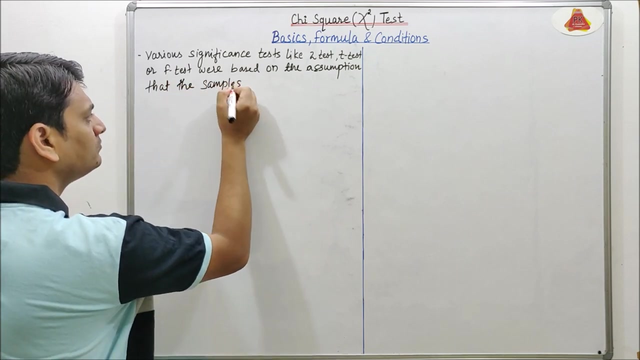 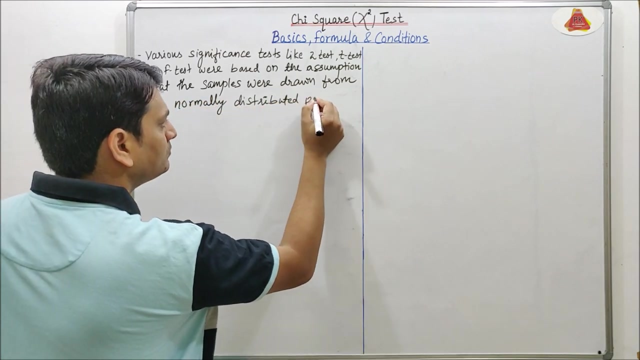 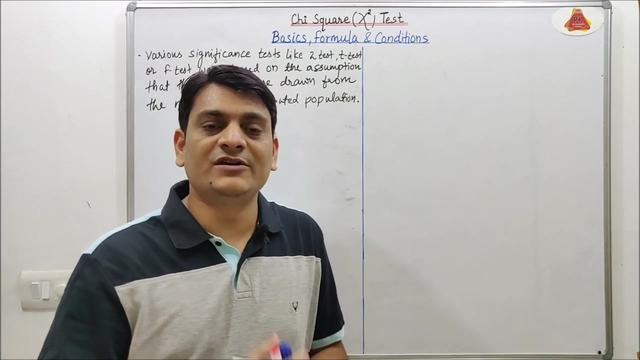 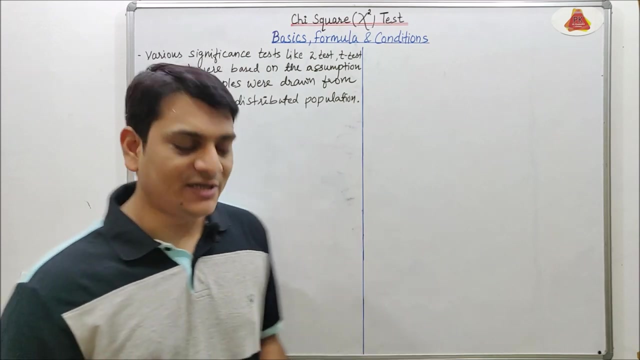 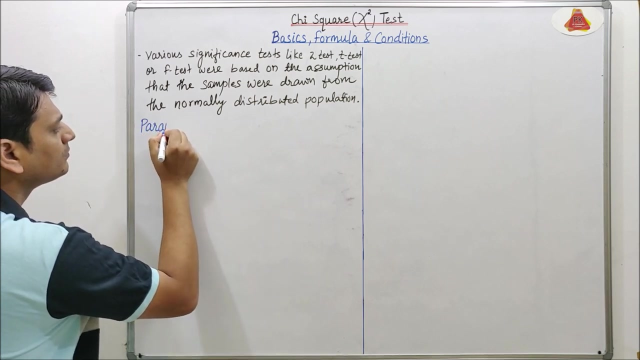 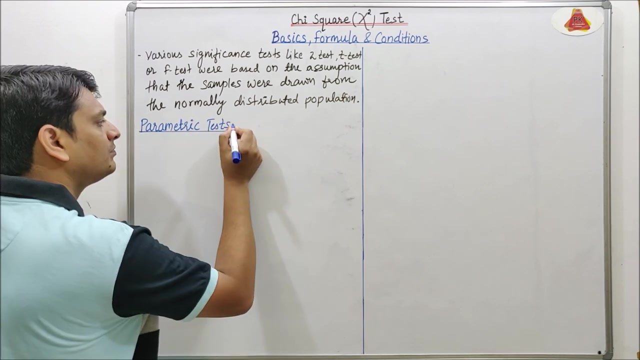 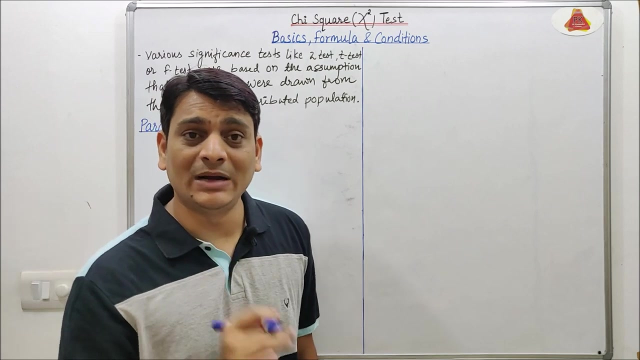 chi-square test. So based on the information available for population. there are two types of tests. First one is parametric test and second one is non-parametric test. So coming to the first one, which is parametric test. So what is parametric test? In parametric test testing process requires assumption about. 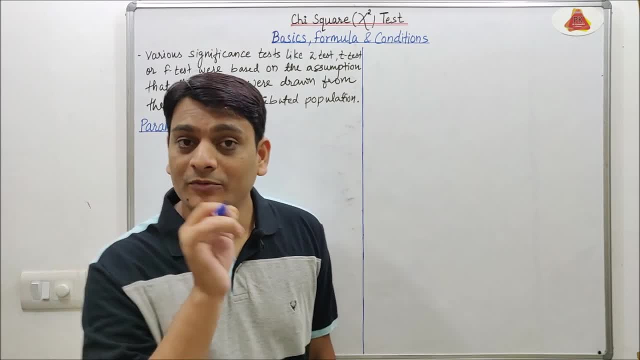 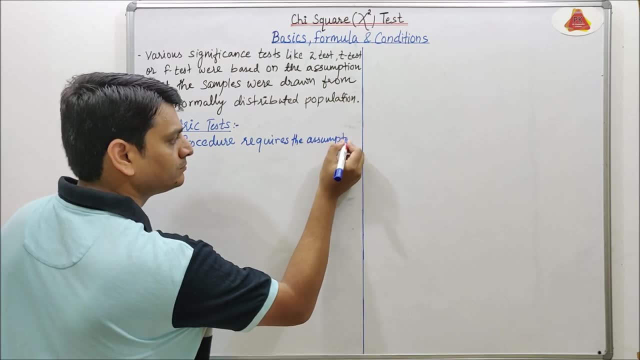 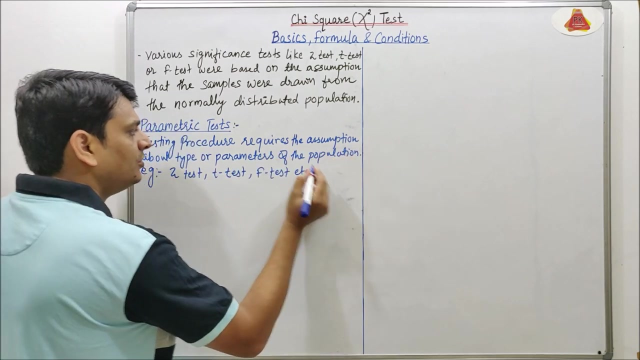 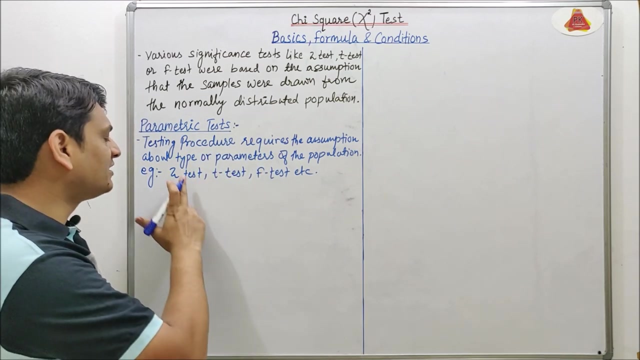 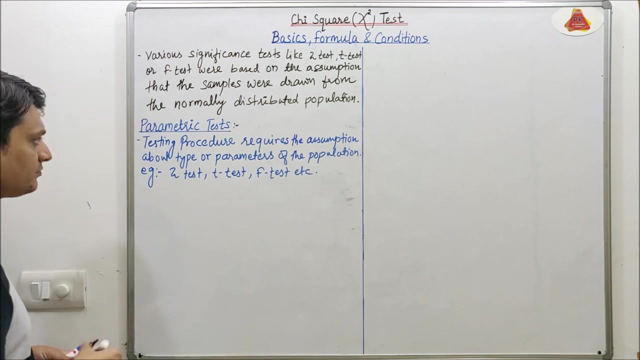 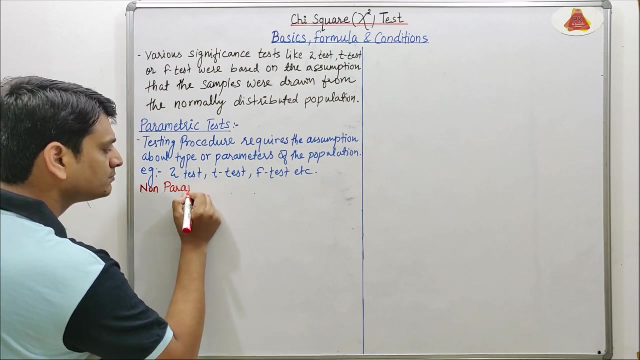 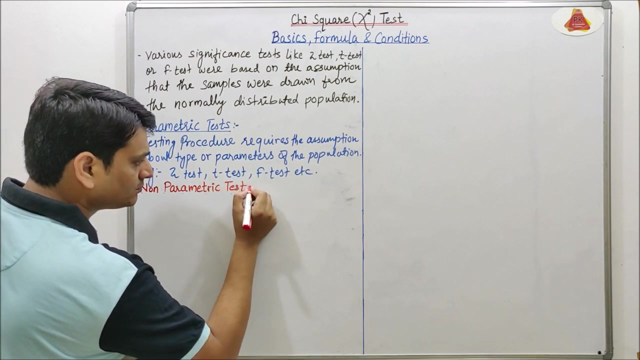 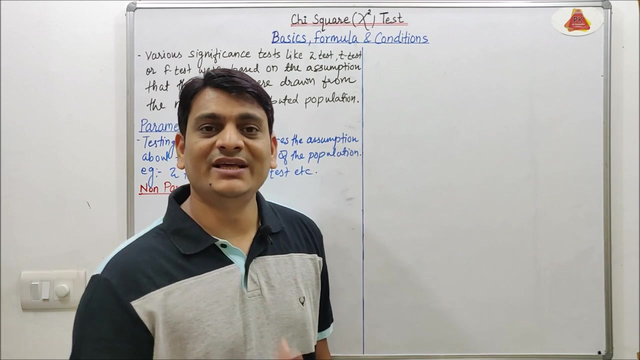 type of population or parameters of the population. So fundamental of parametric test is that we should have information about the population, and example of parametric test are Z test, T test, F test, etc. Now coming to the non-parametric test. So non-parametric test is applied by the statistician when there is no exact information is available. 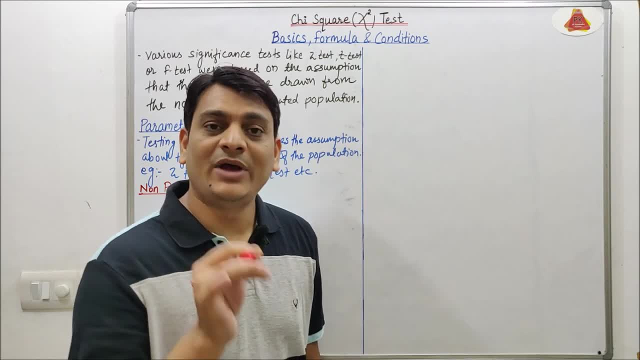 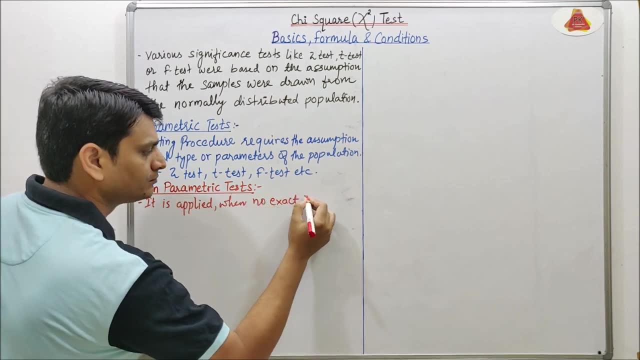 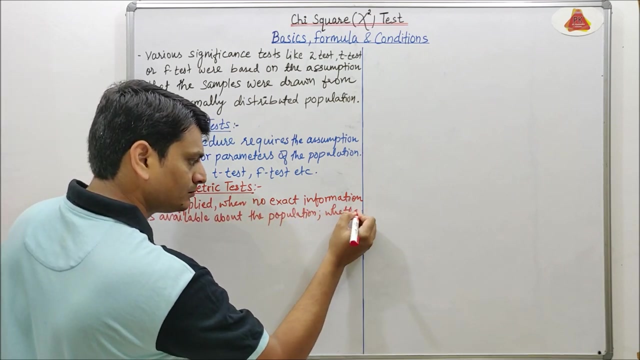 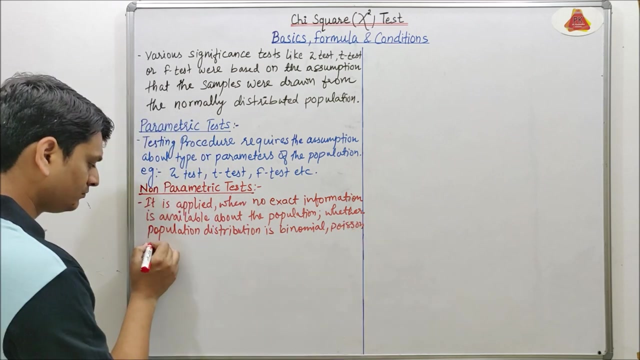 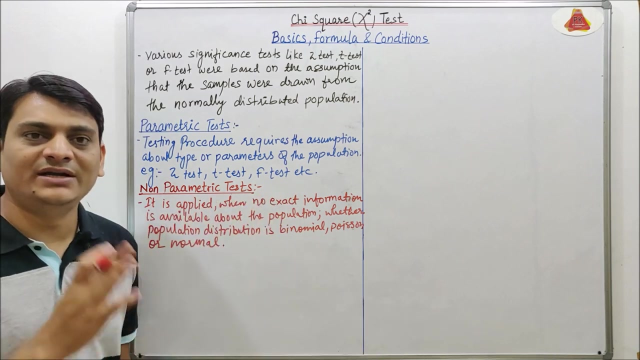 about the population, whether the population distribution is binomial, Poisson or normal. So in non-parametric test there is no information available about the population. that is why this type of testing is also considered as distributional. So in non-parametric test there is no information available about the population. that is why. 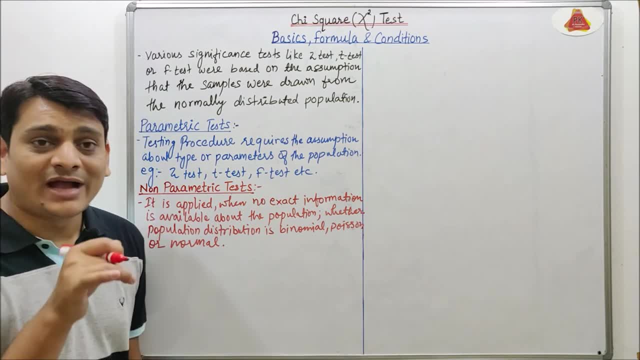 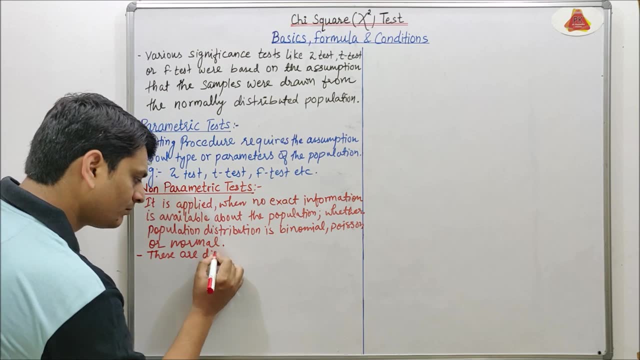 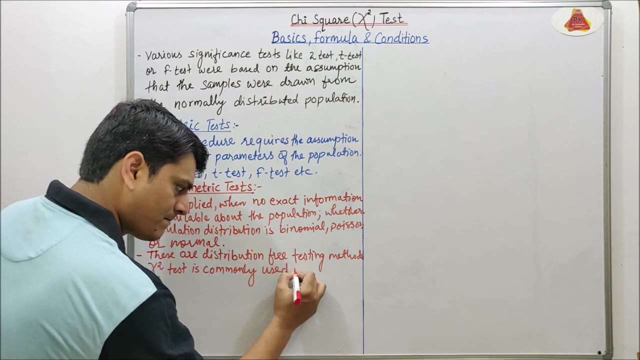 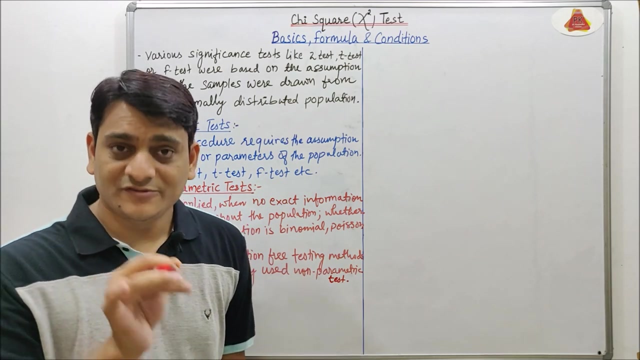 this type of testing is also considered as distributional. So this type of testing is also considered as distribution-free testing, And chi-square test is one of the commonly used examples of non-parametric tests, Step 3.. Now coming to the chi-square test. So the chi-square test was first used by Carl. 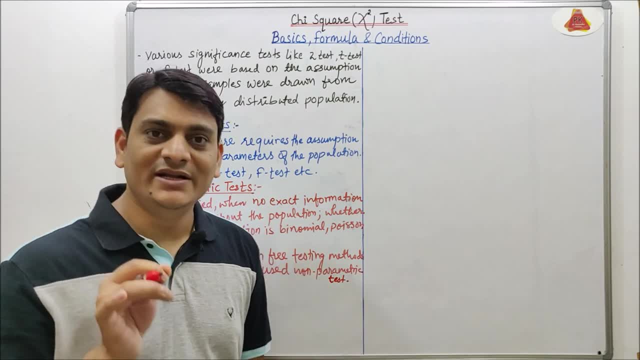 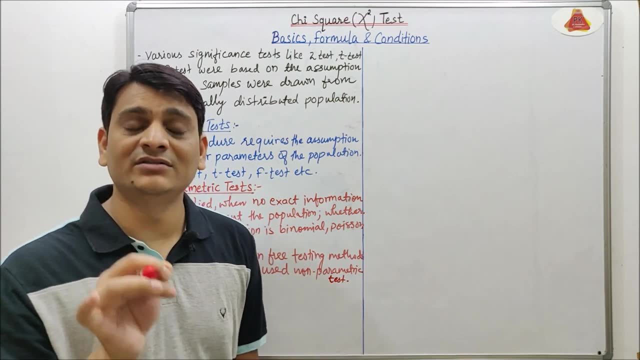 Pearson in the year 1900. Period. That is why it is also called Pi-Square test. So you see its uses base. it is also winner in kg called as Pearson's chi-square test and it is denoted by square of the Greek word that. 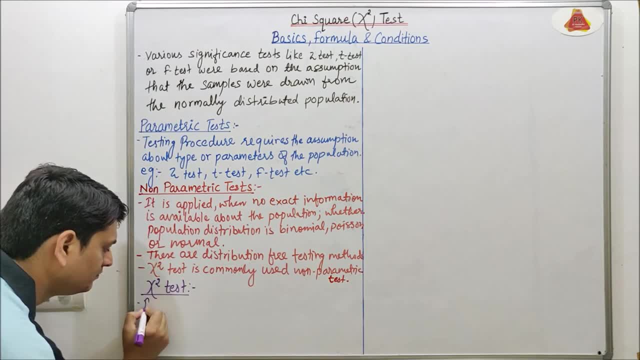 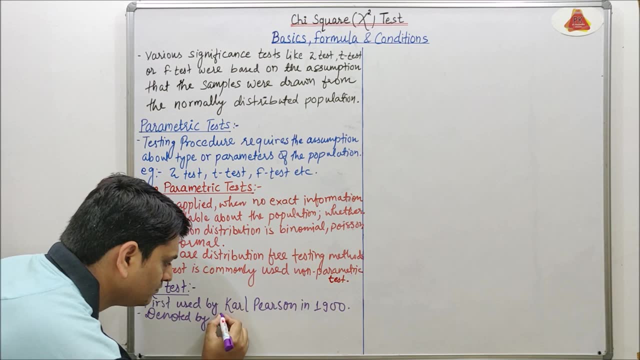 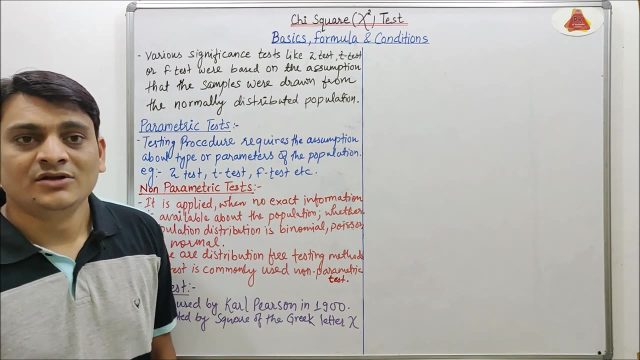 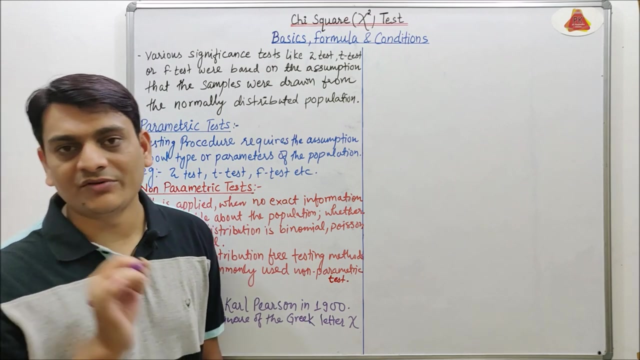 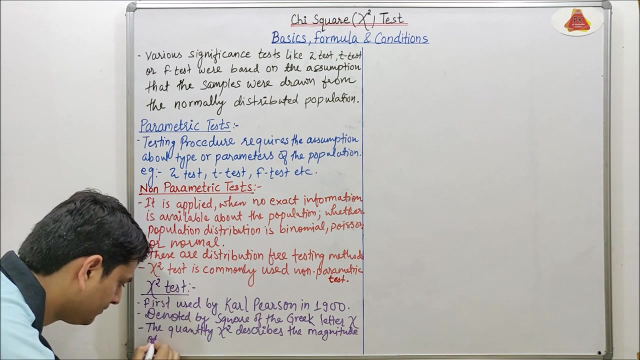 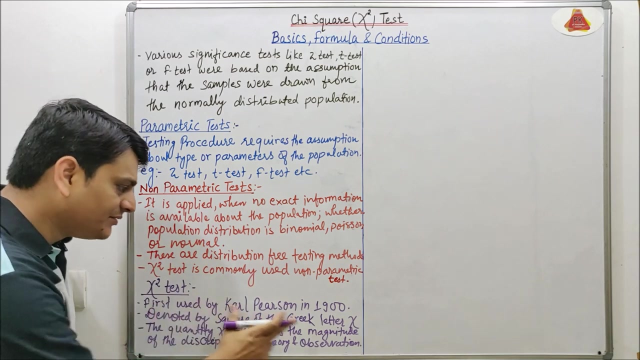 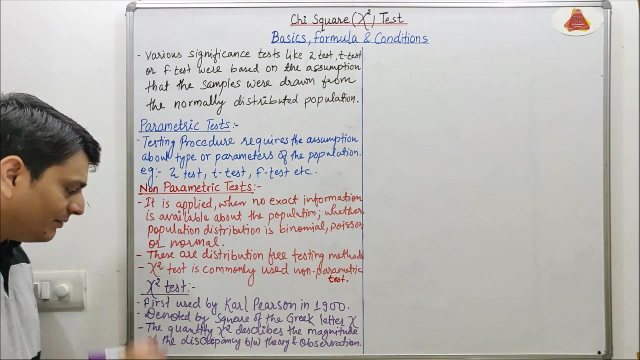 is chi. Now coming to the definition of the chi-square. so the quantity chi-square describes the magnitude of discrepancy between theory and observation. So chi-square describes the magnitude of the discrepancy between theory and observation. It means it will measure the magnitude of difference between theoretical value and observed. 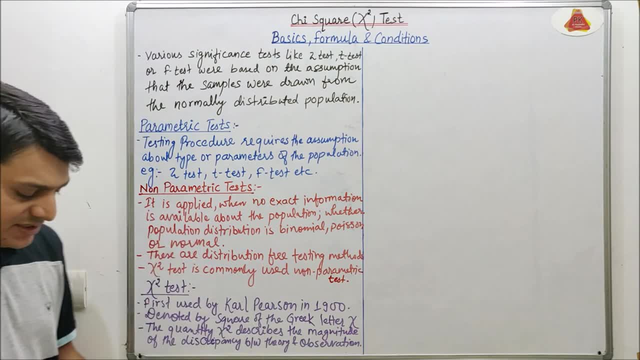 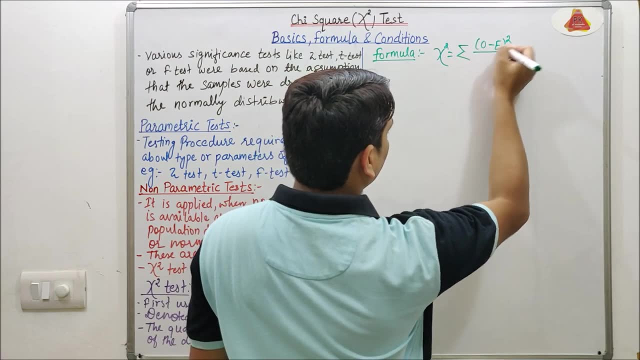 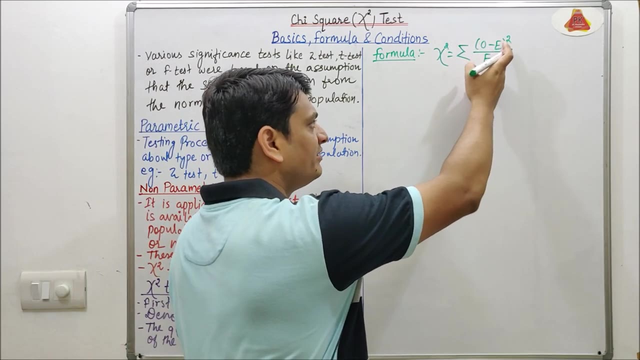 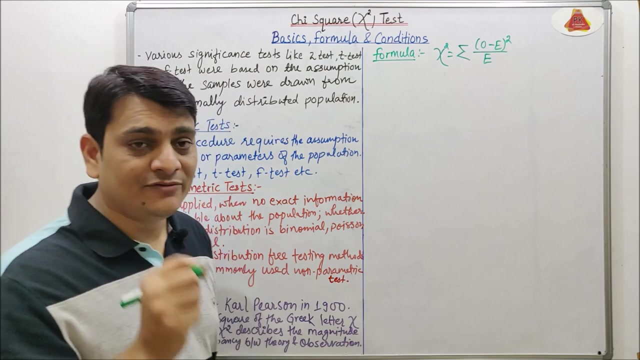 value. Now coming to the formula to calculate the chi-square test. So formula to calculate chi-square is summation O minus E, whole square divided by E. So what is O, O is the observed frequency. What is E? E is the expected frequency. 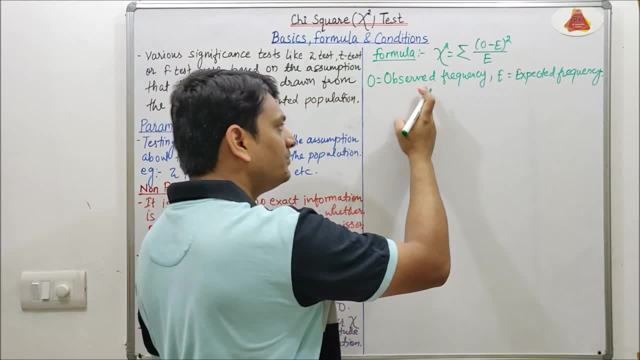 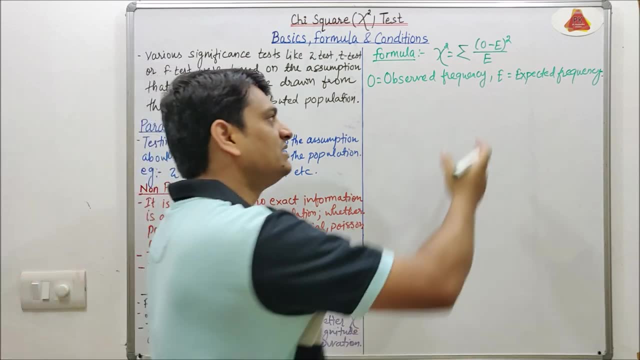 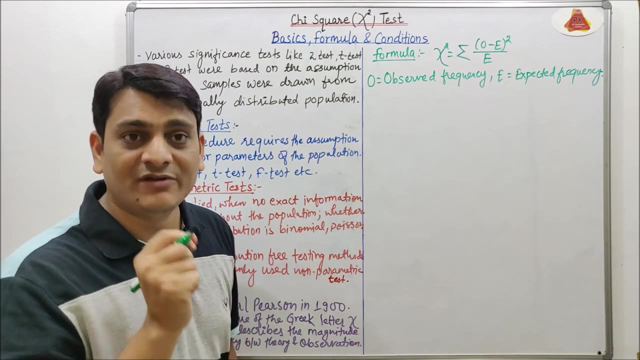 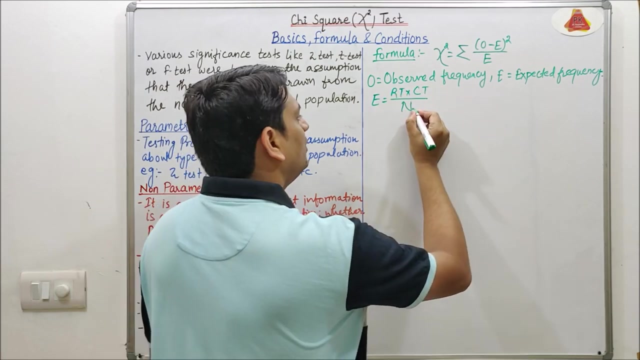 So, as per this formula, O means observed frequency will be observed by the statistician or by the analyst, or if we are solving any question. So this observed frequency will be given in the question. Now coming to the expected frequency. So expected frequency should be calculated by using this formula. 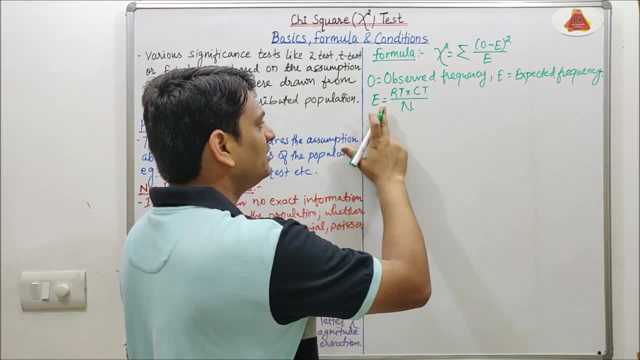 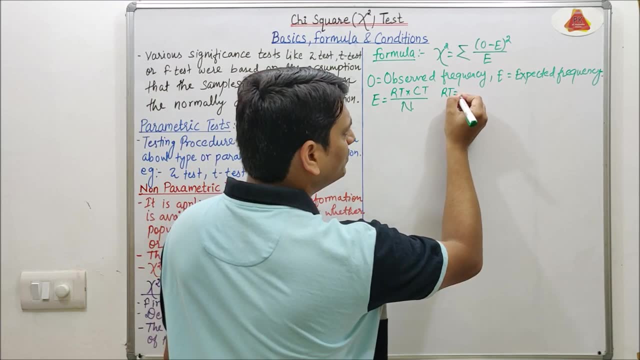 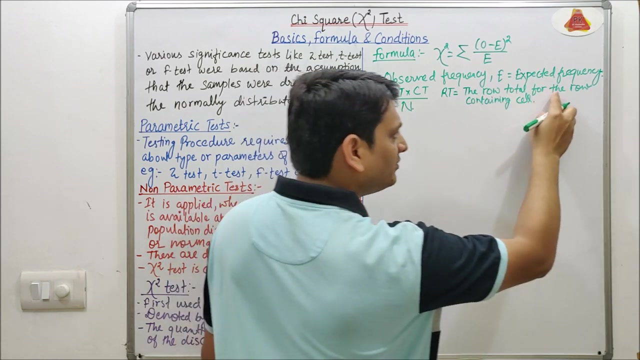 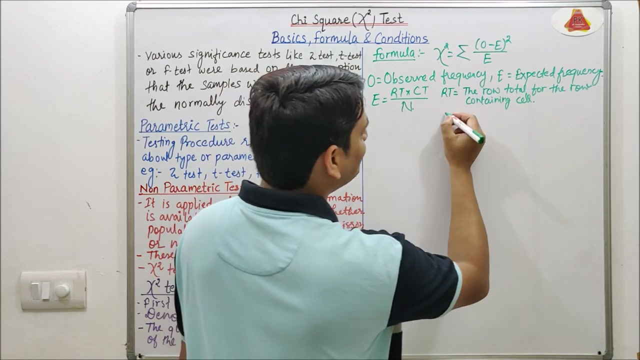 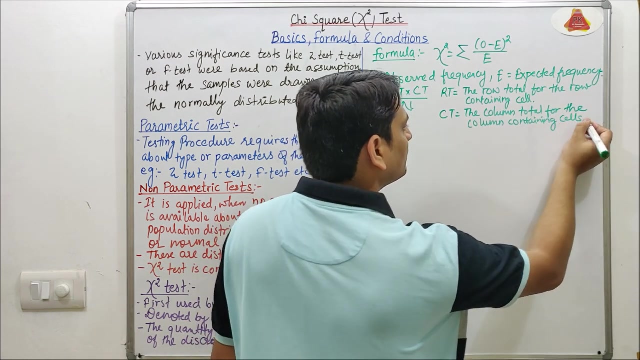 So expected frequency can be calculated by using this formula: E is equal to Rd, Rd is equal to Rt into Ct divided by N. What is Rt? So Rt is equal to the row total for the row containing cells. What is Ct? Ct will be the column total for the column containing cells. 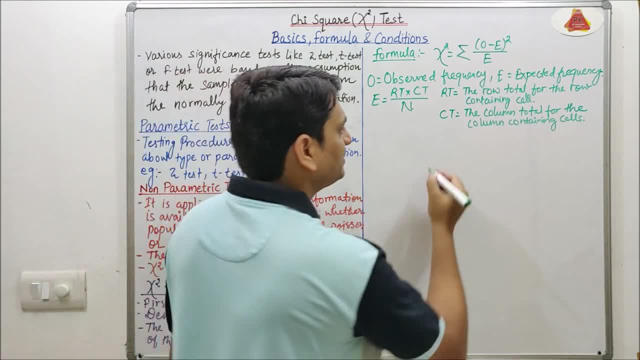 And what is N? N is the total number of objects. What is Rt? N is equal to N And what is the given value of O? Rt is equal to RtR, So this is the value of O given for the question. 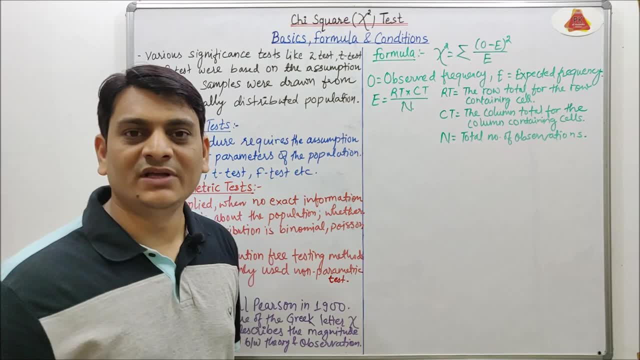 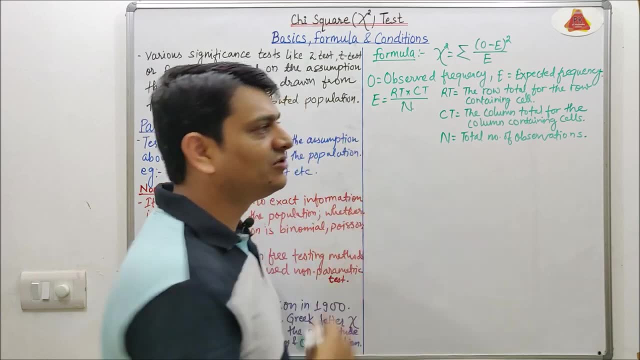 So the value of O is calculated by using this formula. So by using this formula we can calculate the value of chi-square. The value of O will be given in the question and the value of E is calculated using this formula. Now coming to the degree of freedom for chi-square test. 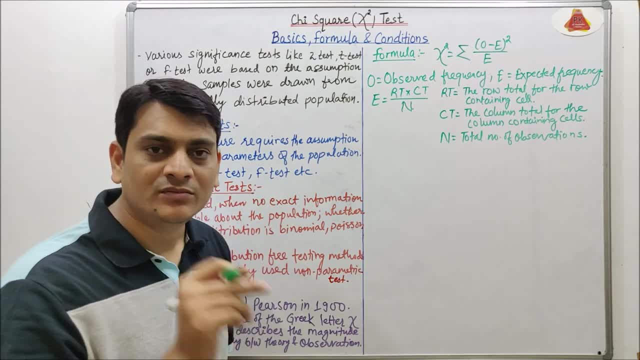 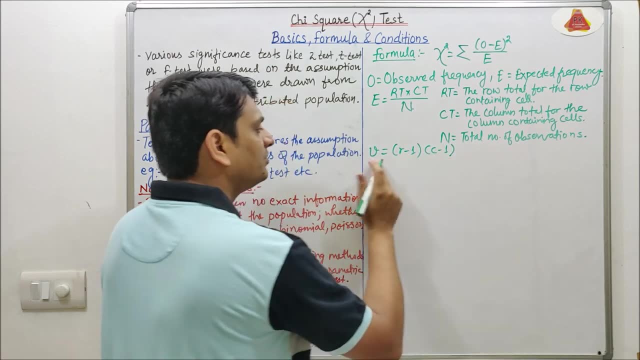 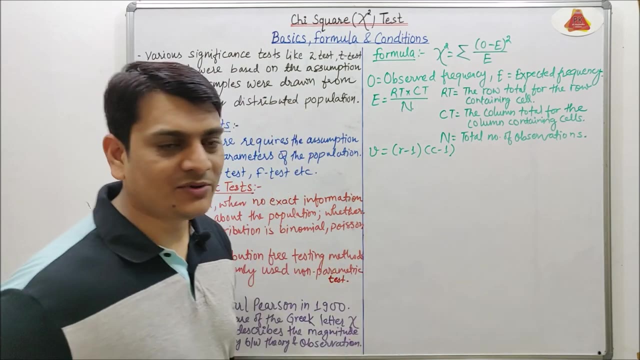 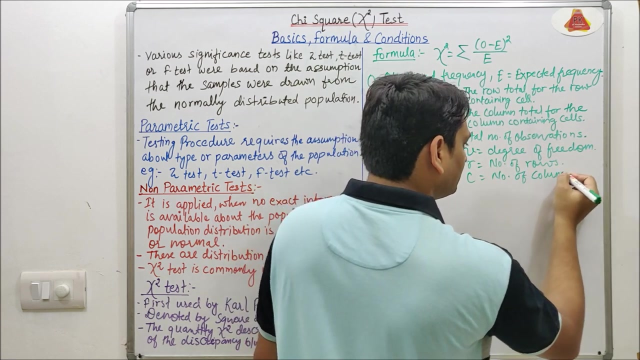 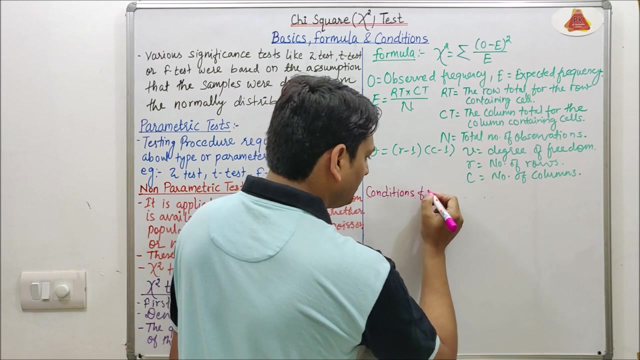 So degree of freedom or nu is equal to So, in this formula, nu is equal to degree of freedom, r is equal to number of rows and c is equal to number of columns. Now coming to the conditions for applying chi-square test. 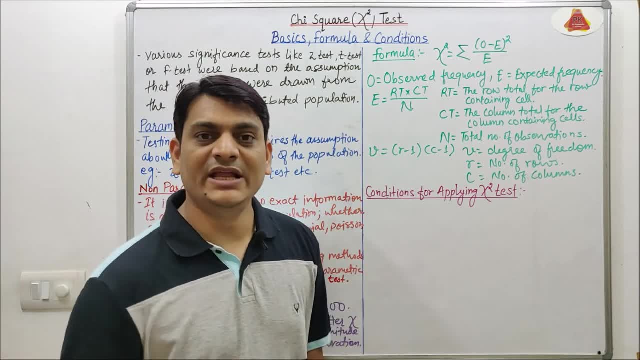 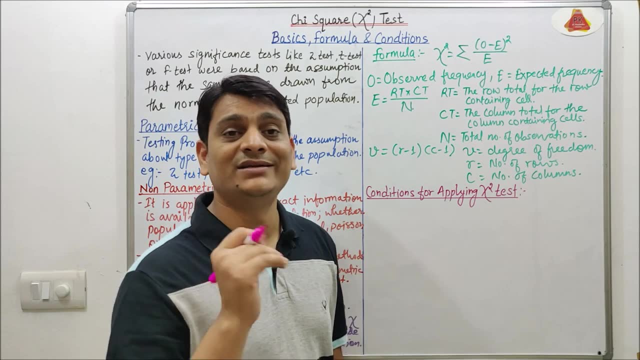 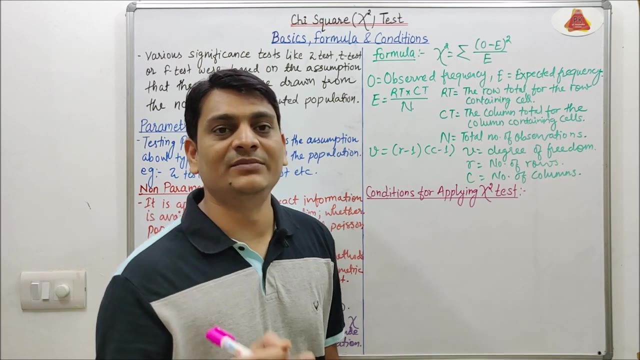 So coming to the first condition for applying chi-square test. So each cell should have minimum of 5 observations or 5 observed value. Sometimes it is taken as 10 observed value. So if observed value will be less than 5, in that condition chi-square will be overestimated.